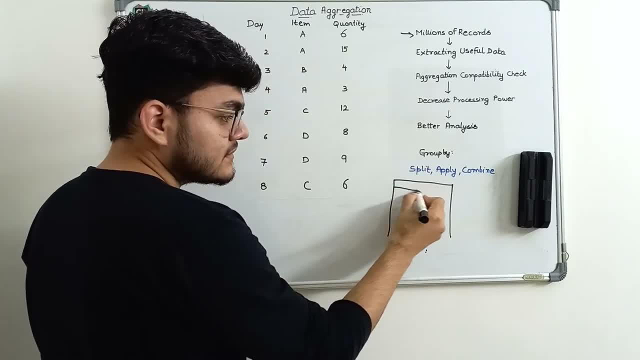 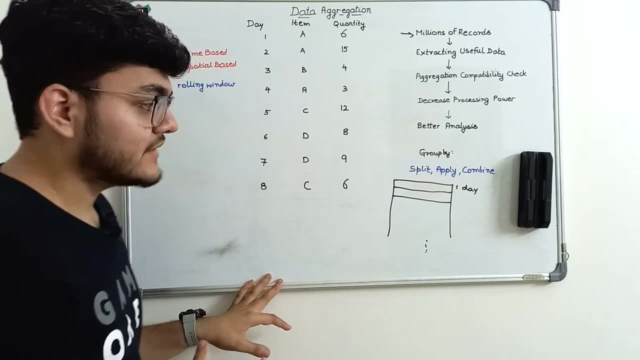 And it has millions of records in it And let's assume that each and every row in this data set represents one day of sales that happened, right, So during one day, the number of sales that happened- let's assume here it is 28.. 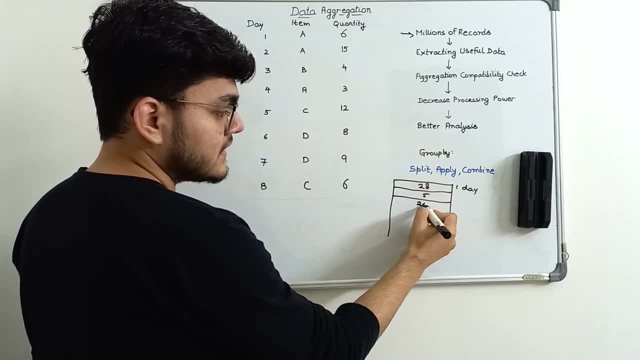 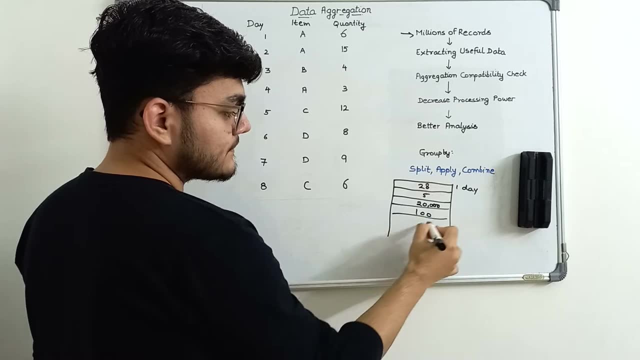 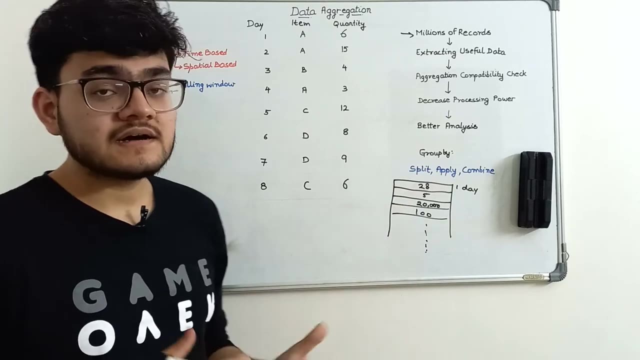 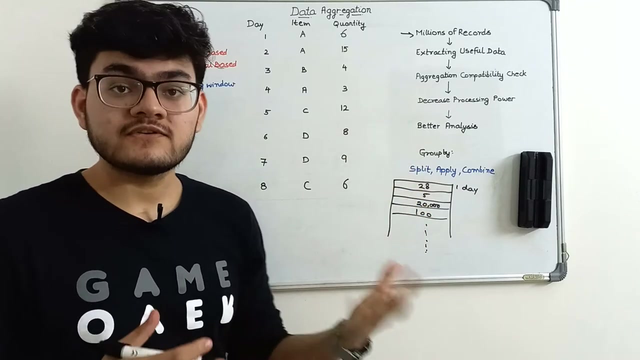 Here it is five, Then Let's say 20,000.. Some days were like 100 and so on. right, So every day different numbers are being chosen here You can see, because sales are not actually predictable. They are going to. sometimes, if the company does marketing, they will have a good sales, and some days are like they will have lower number of sales. 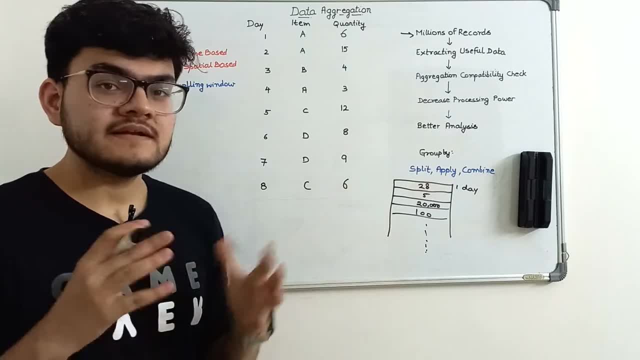 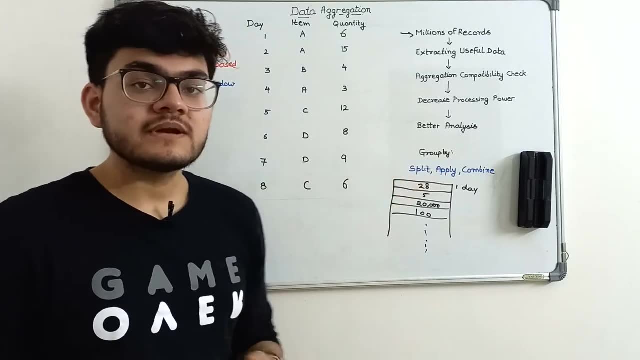 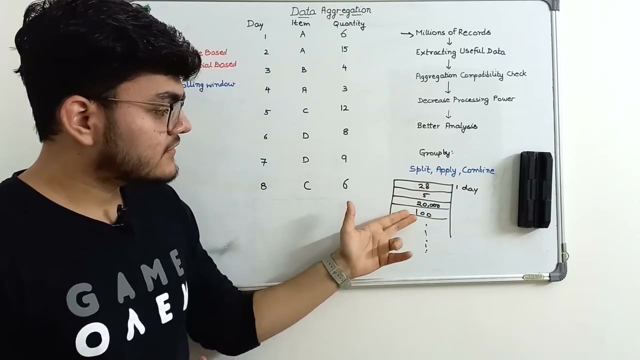 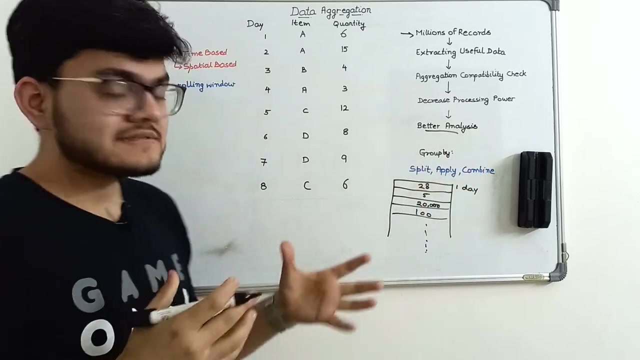 So you can see that, if I have a data set, Let's just imagine that you are a data scientist and you are given a data set which is where each and every row represents a single day of how many sales happened during that day. Now it becomes very difficult because if you try to plot this on graph, if you try to analyze this, which is we want to analyze it, why do we want to analyze it? 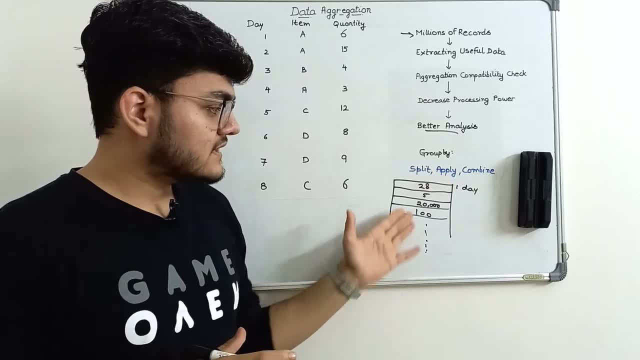 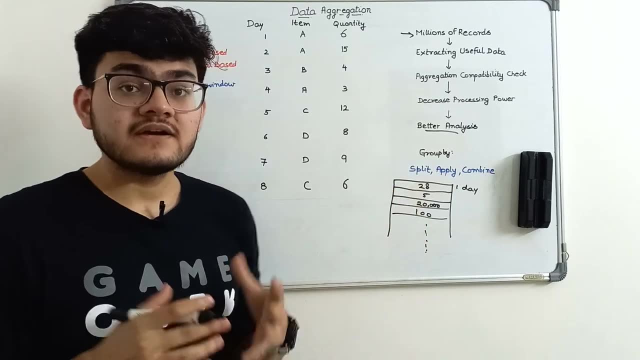 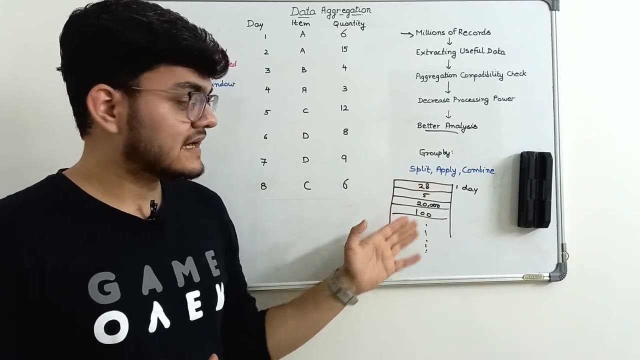 Because there is a business requirement. But now you can see it is very difficult to analyze this type of data set Because the values are so much you can see there is a higher difference in them. So if I take an average and then I calculate the standard deviation, you can see that the standard deviation will be very high in this case. 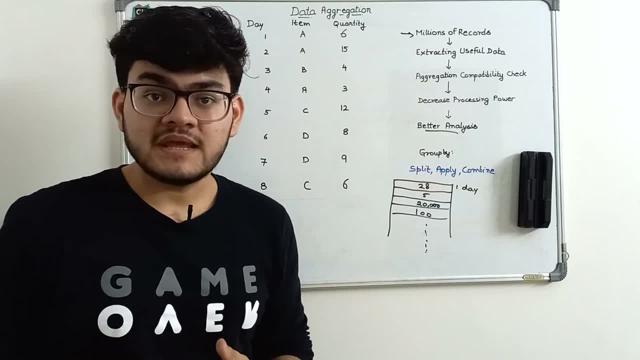 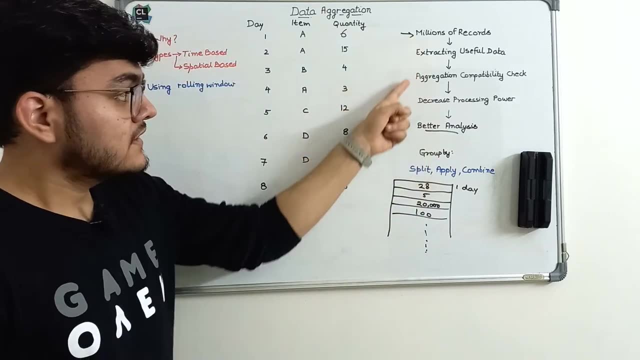 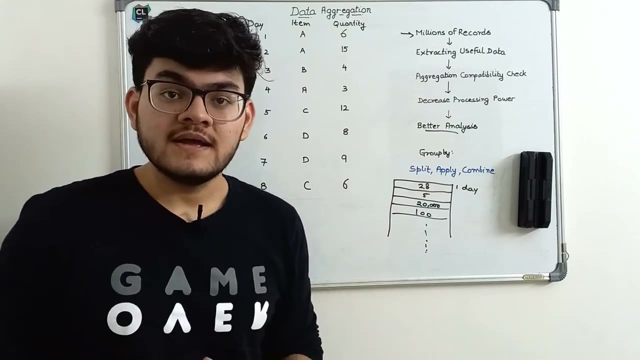 Right And it is because they're going to deviate a lot from the mean Right. So exact data and analysis will become difficult And there are millions of records So it will also take a lot of processing power to actually do The analysis of such a big record. 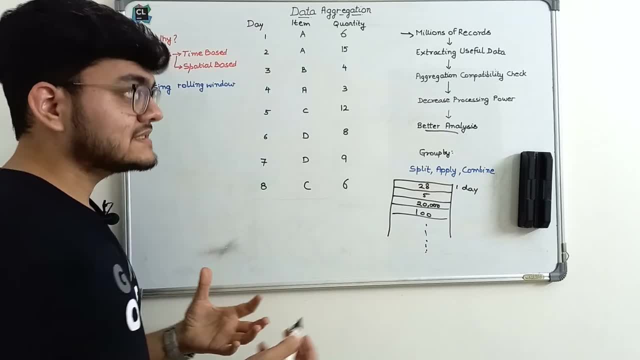 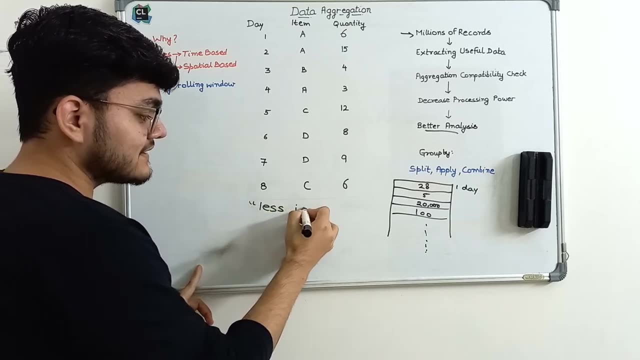 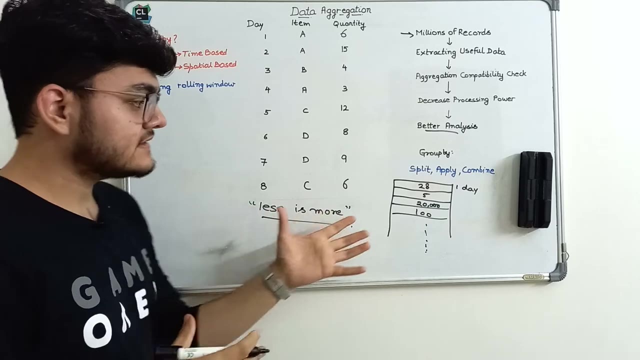 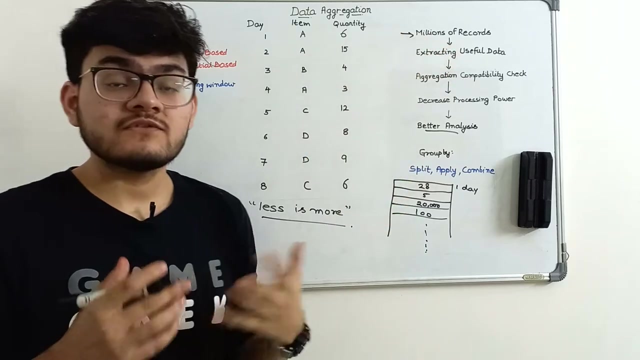 So there is a very simple technique which is very important, and it is the data aggregation technique, And it actually justifies this very simple thing, which is less is more. So less is more means that the less information if it is useful for a business, it is actually more so, instead of having millions of records that do not actually give us some. 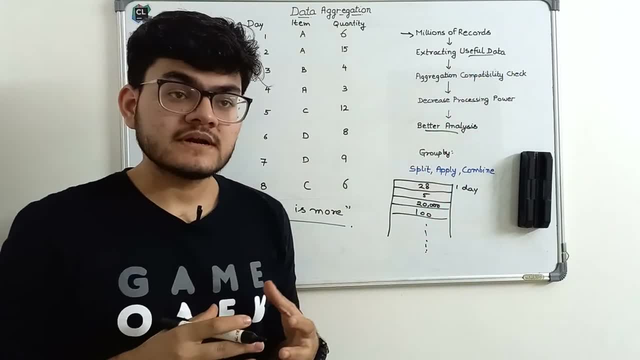 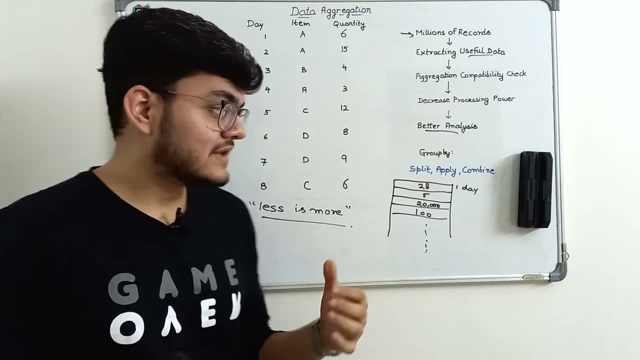 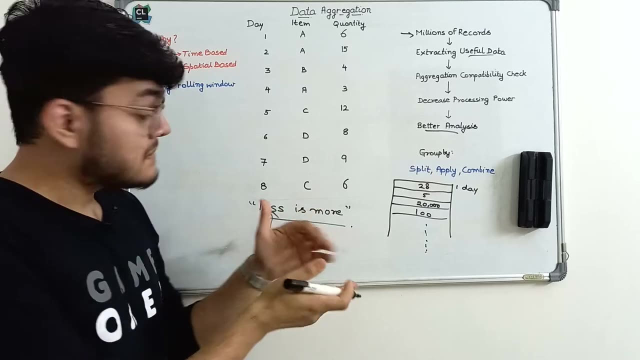 use Well data, some useful information about the data, then it is actually a not good idea, Right? So what we want to do is we want to use some techniques so that we can actually make this data set much shorter, which means we want to make it lesser. 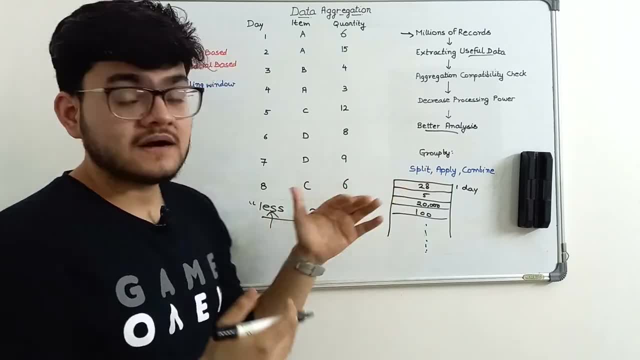 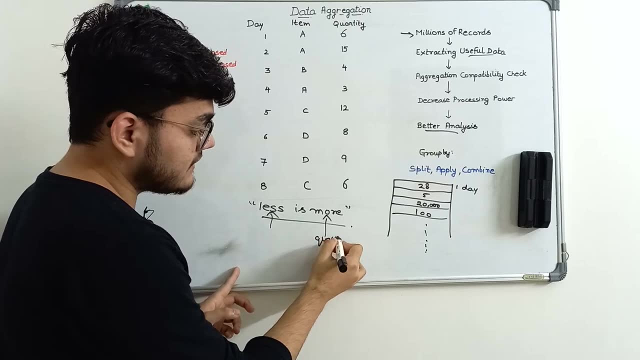 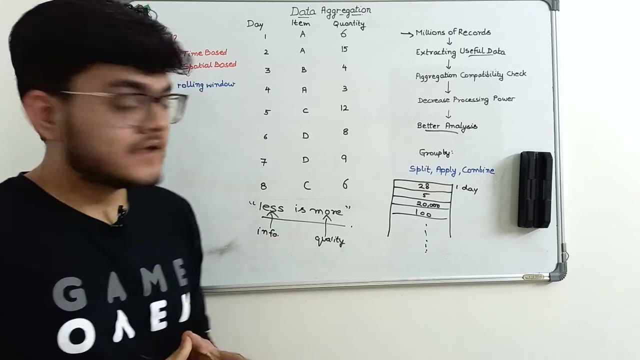 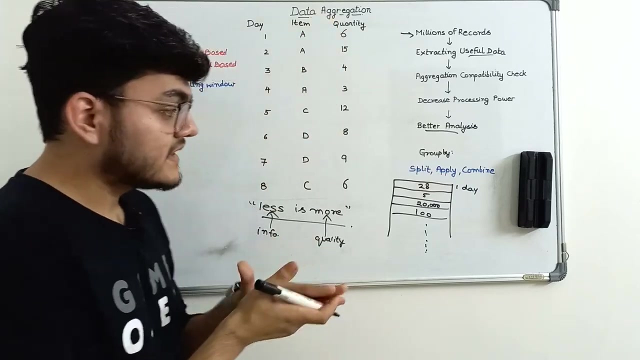 But at the same time, we want to increase the quality of information that it holds, which is, we want to increase the quality, Right? So here we are going to increase the quality And we are going to decrease the information, Right? So this is what data aggregation does. as the name suggests, data aggregation is actually aggregating or groping the rows. 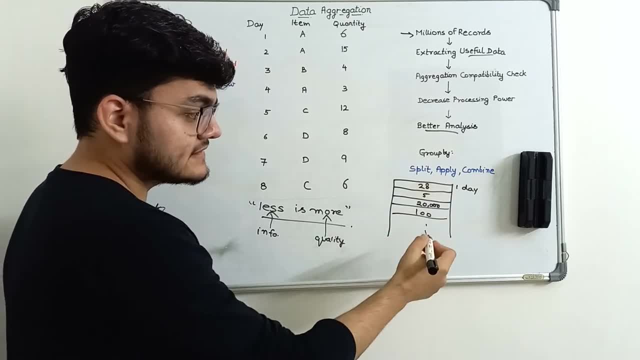 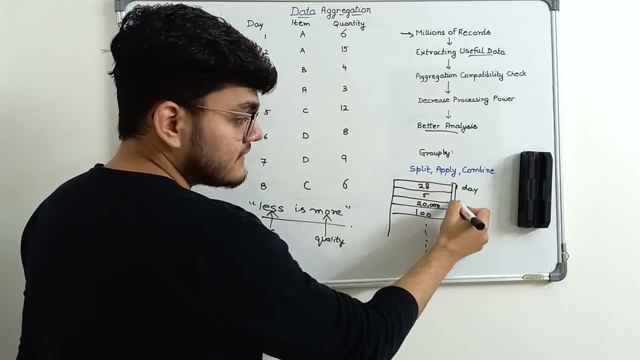 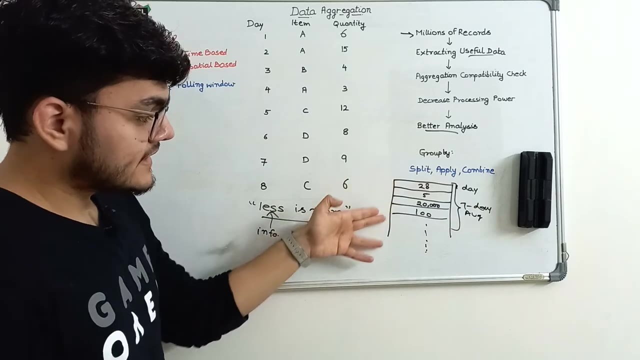 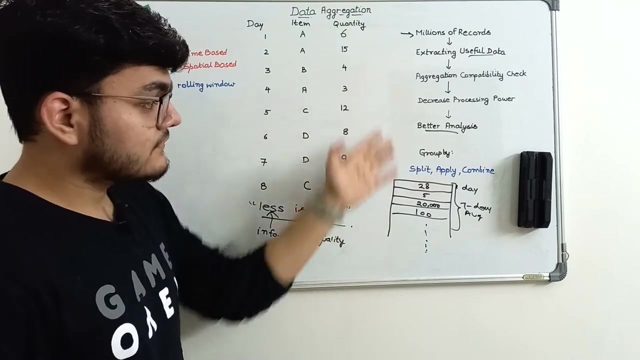 Now, let's say that we have these sales now, instead of using everyday sales. what I can do is I can actually pick up seven day average. Right, I will pick up seven day average And I will take seven days, All the values. I will take the average and I will combine them in a single row and I will do that so on with the millions of records, and then you will observe that the data is now lesser. 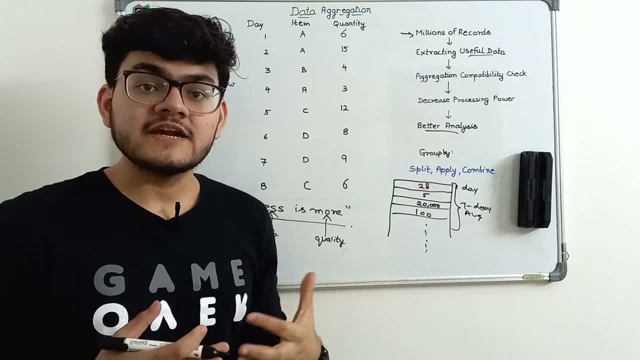 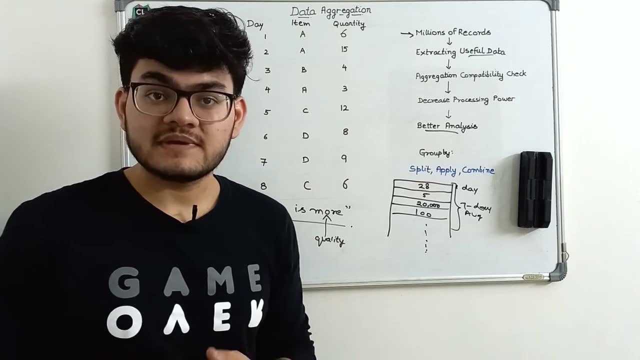 And if you try to do the analysis, maybe it is- it will give a much better analysis, Maybe it will give a graph that is much useful for a particular business. So that is very important in data aggregation, which is we want to minimize the data set. 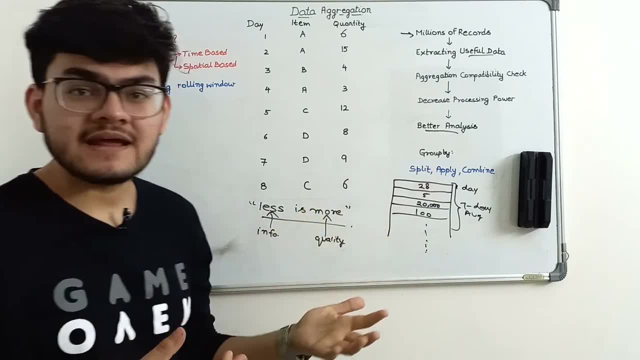 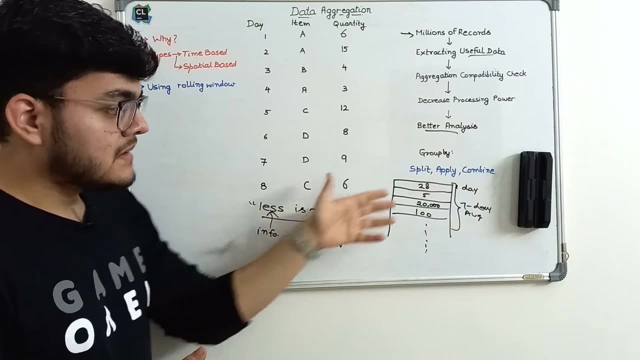 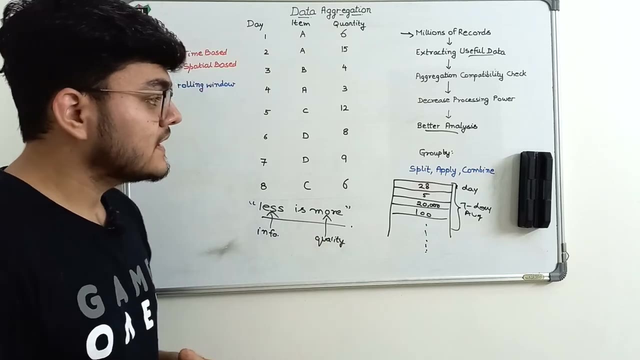 We want to do something, Use categorization or something to actually merge the rows, which is actually making the information lesser, But we also we also want to make it give more quality information about the data. So let's take a very good example here that I have taken. 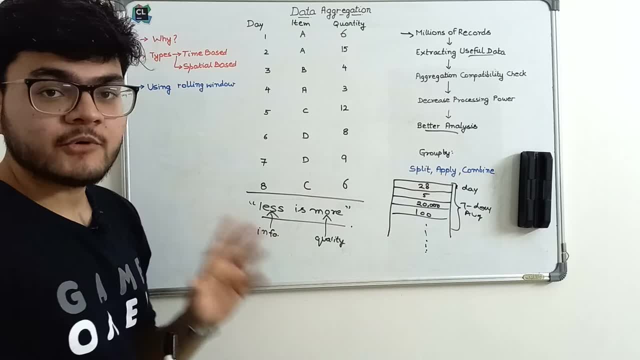 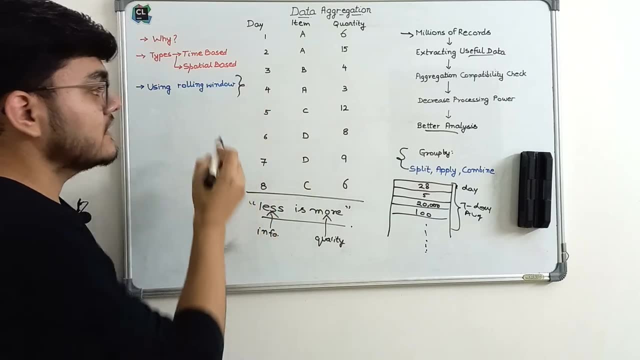 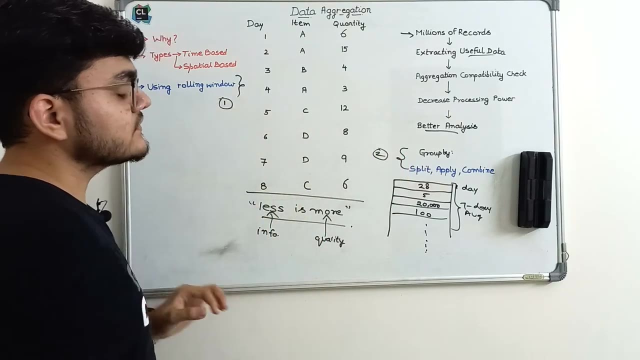 This is. there are basically two important techniques which we will implement in Python. One is the group by technique And the second one is the Yes Use of rolling window. So these two techniques are very important and I've personally used it in a lot of projects. 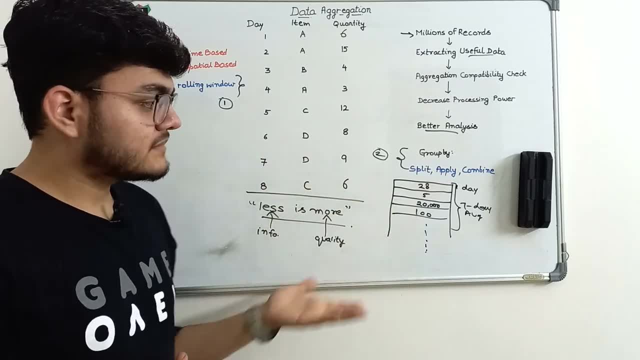 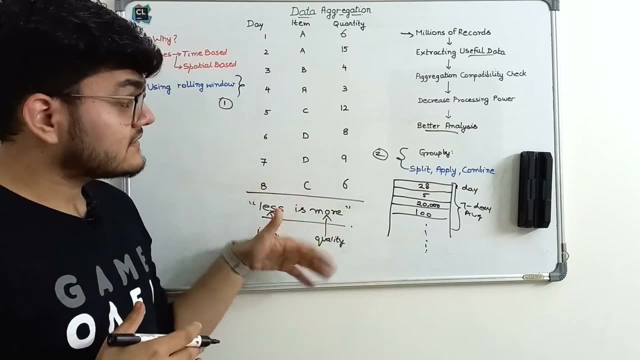 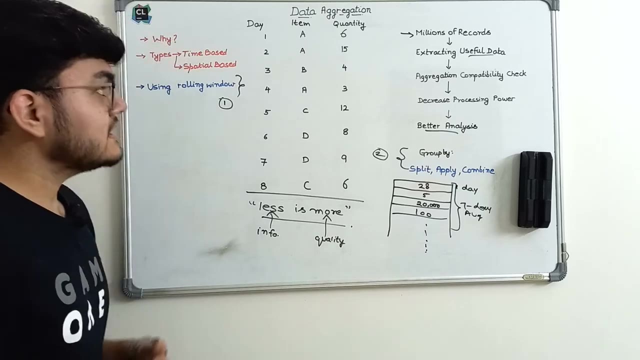 There are various techniques to perform data aggregation apart from these two techniques. So, basically, data science is a very creative task. as you will understand these basic concepts, You will come up with your own techniques of aggregating or merging the rows right. So, basically, data aggregation can be your time based or spatial. 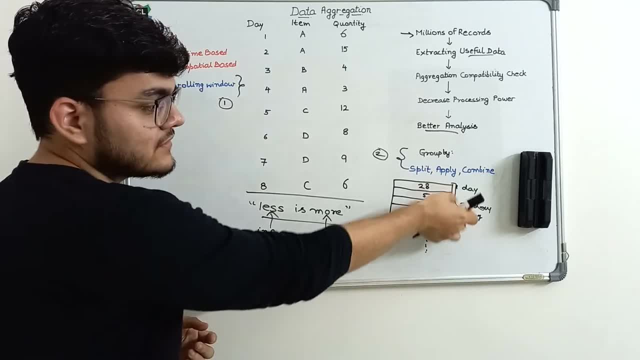 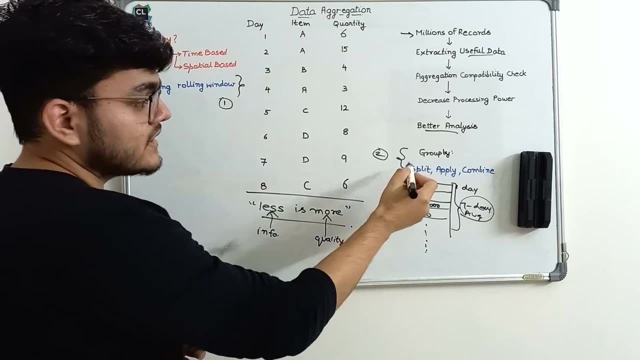 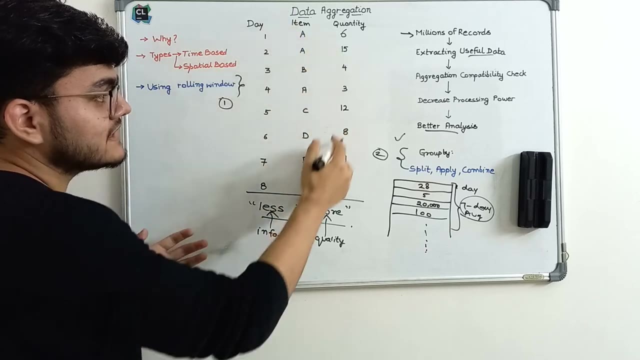 Based. so time based means you're actually merging the rules on the basis of time, that I'm taking a seven day average or something like that. Let's understand the what is the this group by so first we will understand this technique group by right. So let's suppose we have this data set where I have the number of day. 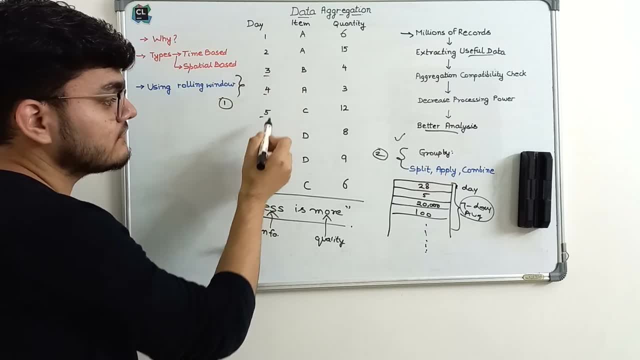 So one day, one day to day three, four, five, six, seven, eight, right? So this is the data set that is given to me and these are. this is the name of the item. So, this is the data set that is given to me and these are. this is the name of the item. 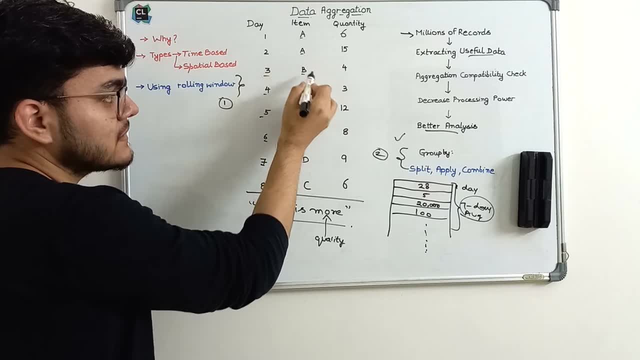 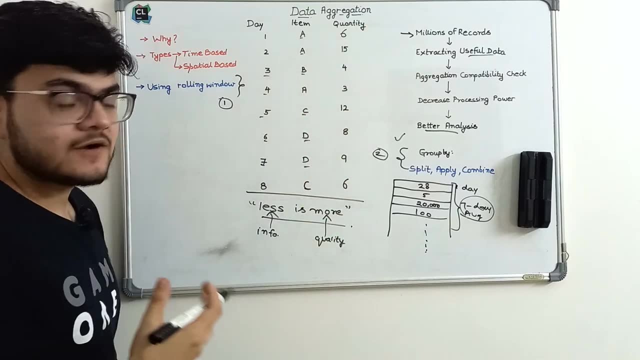 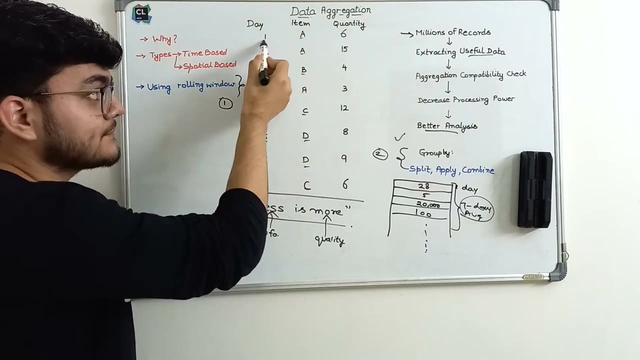 A. so you can see here We have a, a, b, c, d, d, c, right? So we have the item name here and here we have the quantity of these items, right? Let's say, this quantity represents the number of items that were sold during day one. 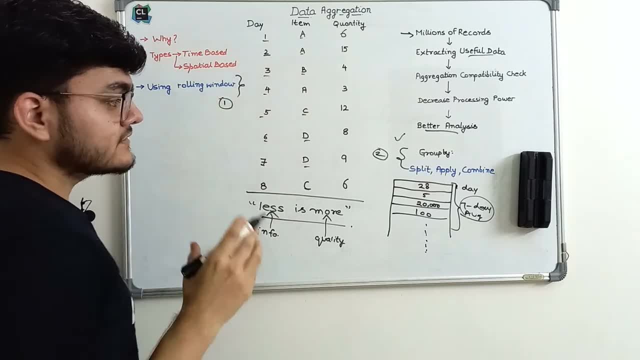 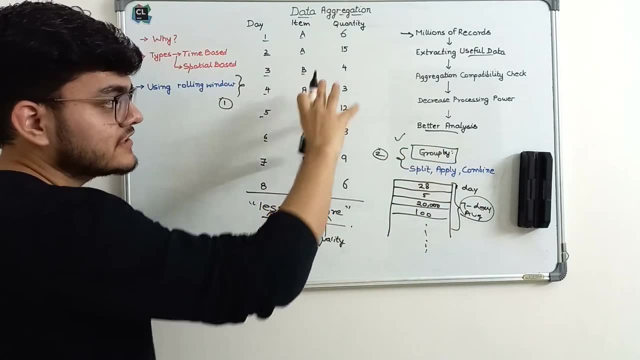 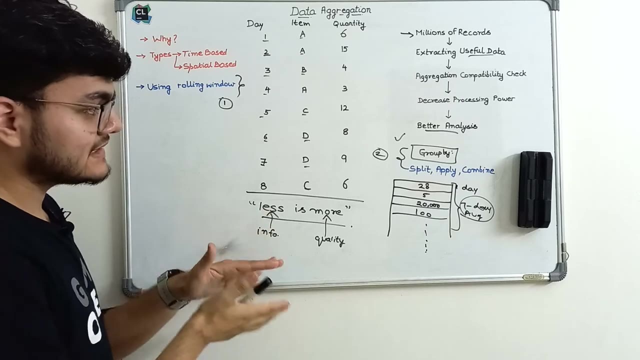 And then during day two, then three and so on. right, So now what I'm going to use is: I'm going to use group by To actually make this data shorter. Right, because our target is to make to minimize the information, to make it lesser, but also increasing the quality. 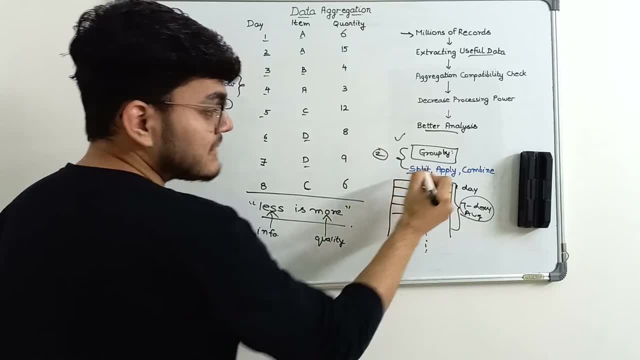 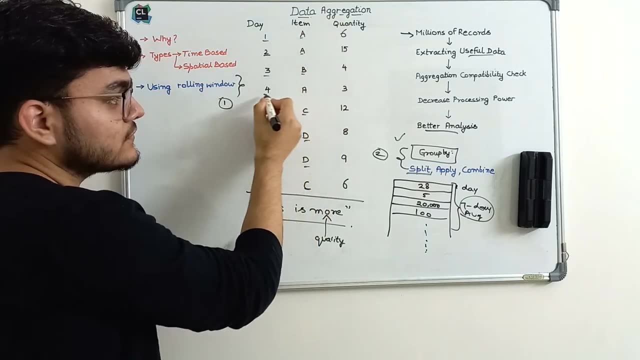 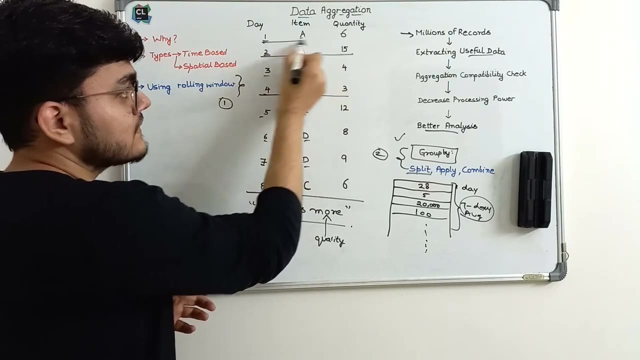 So let's see how we can do this. The first task is to split the data set right. and how we can do that. We can simply take out all the rows which has same item in it, right, So you can see that this row, this row, this row, right? 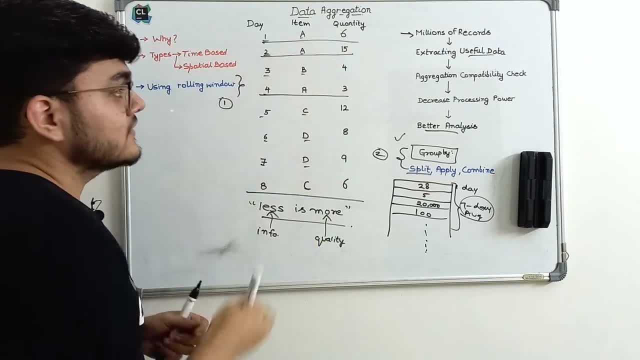 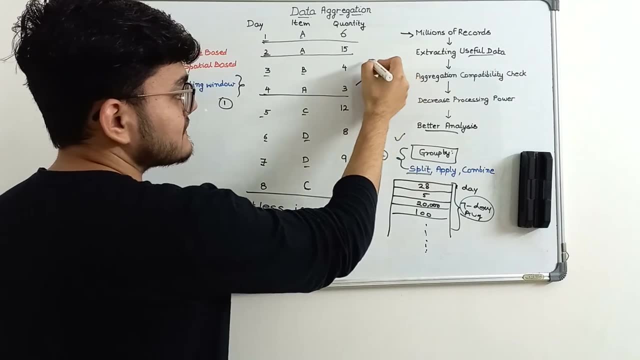 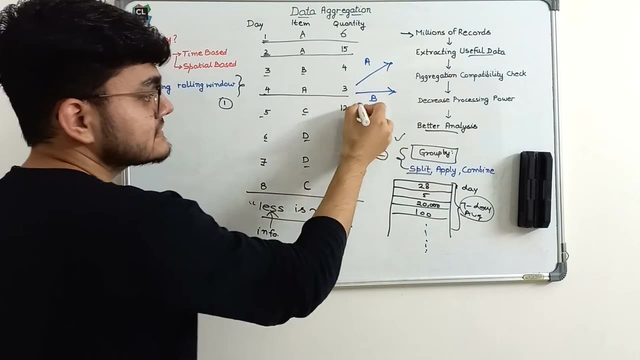 These three rows are Only having item a. so what I would do is I will split this data set, this whole data set, into three ways: One, which has only item a in it. second, which has only item b in it. third, which has only item c and then d, right. 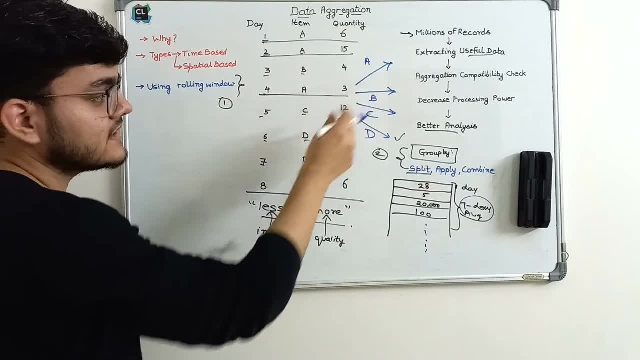 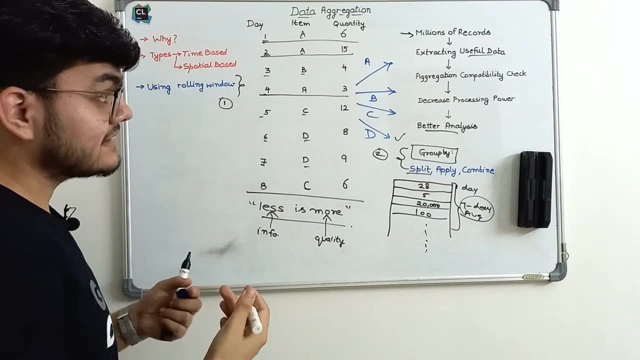 So let's see, if I try to split a, what are we going to get? actually, we are splitting this whole data set into these four categories. So this is Actually categorization. So if I will split this into a, what I'm going to get is: 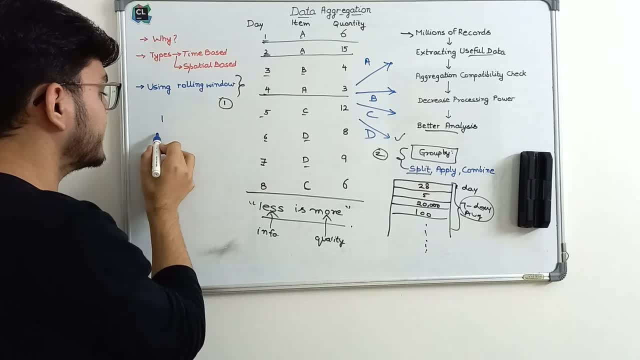 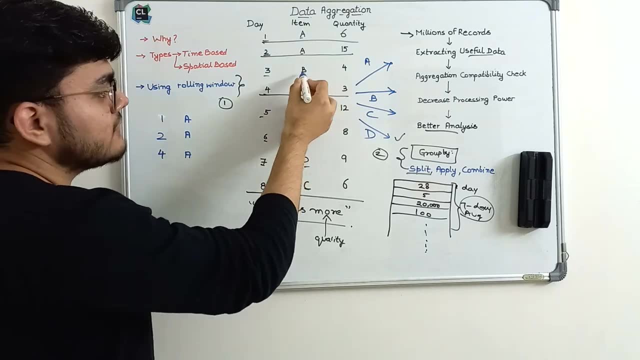 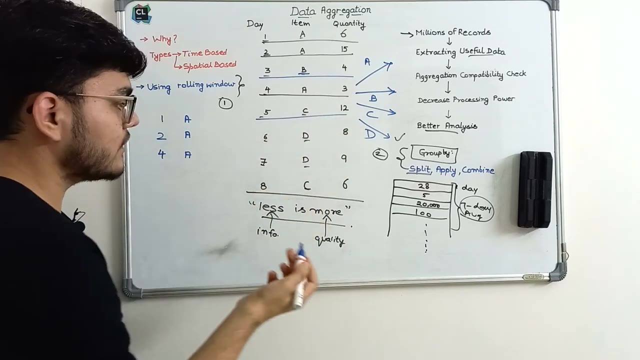 One, Then we have the row number two, then we have four, and these all are a Right. so this is a. now we have b here, Then we have A c here. c has these two rows, and so on. so here we have the quantity as six. 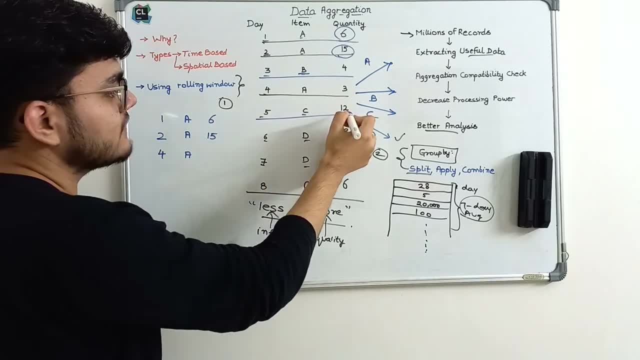 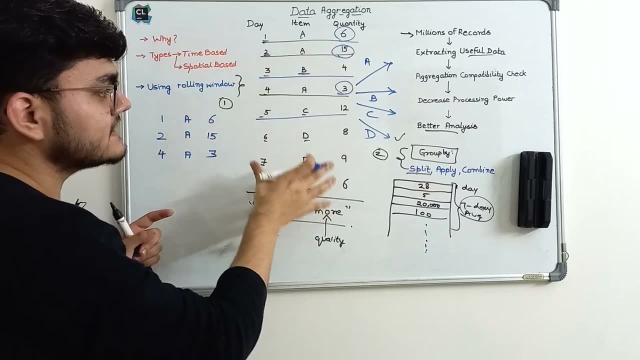 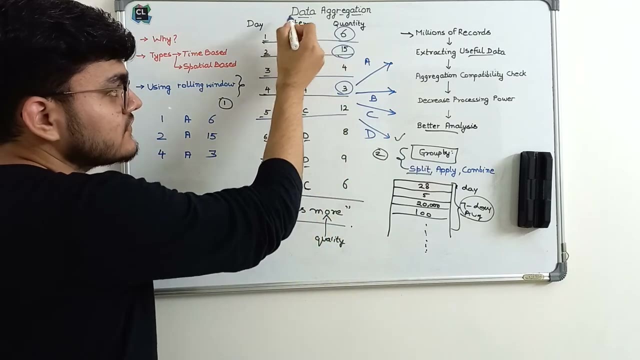 Then we have here Fifteen And finally here we have three. Right, so we have. what we have done is we have essentially divided this whole data set into four categories according to the number of items. So here I have chosen this feature item, right? so I'm using a feature to actually do the splitting. 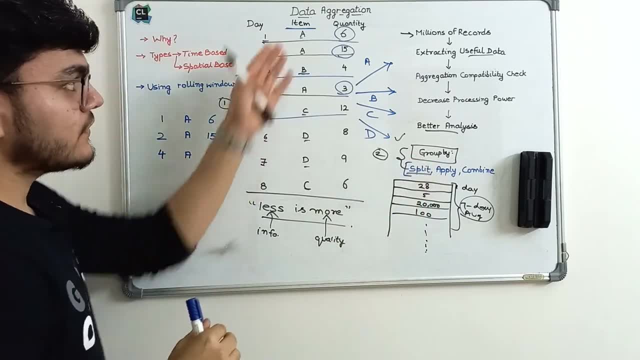 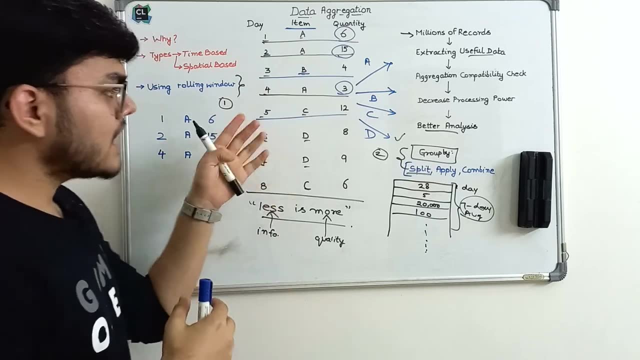 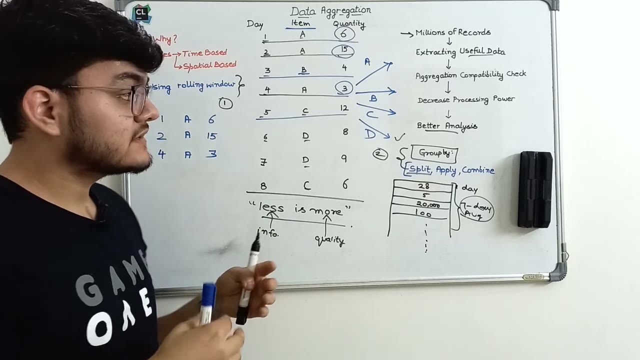 Right, it is very important because we want to aggregate them. So first, what we do is we try to understand what is the Basis of splitting. How can we actually split the rows? because if we can actually convert them into categories, We can do a lot of things with it. we can actually create clusters, we can actually perform some of the aggregation task. 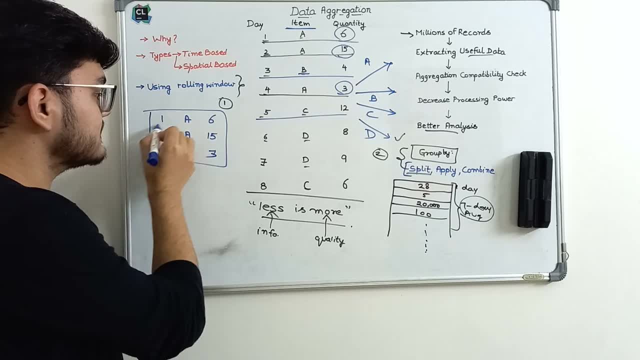 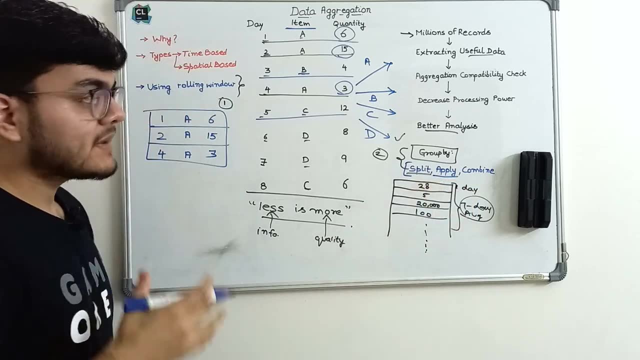 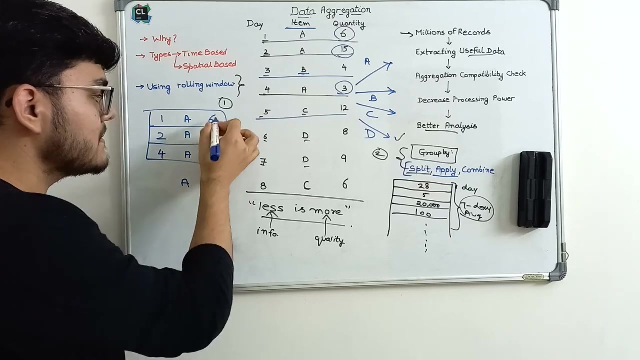 So let's suppose we we have splitted this and now we get this as a subset Right. so now what we will do is we will do the second step, which is apply. apply means now we want to apply the aggregation to this. so what I Can do is, at this step I can actually use different strategies to combine these right. so what I can do is I can combine all of them in a single row. 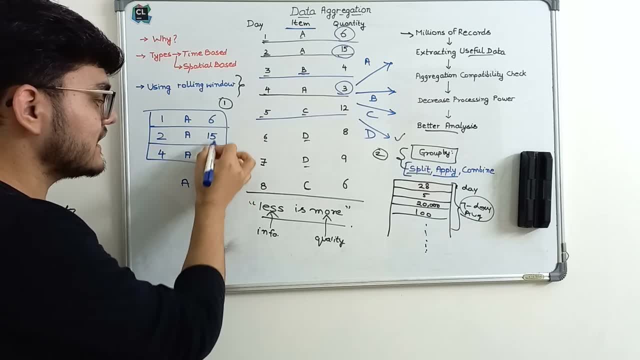 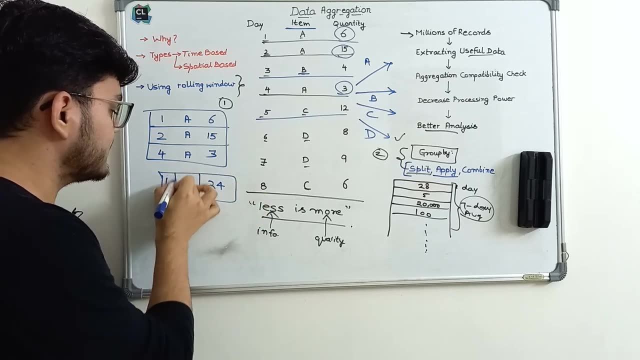 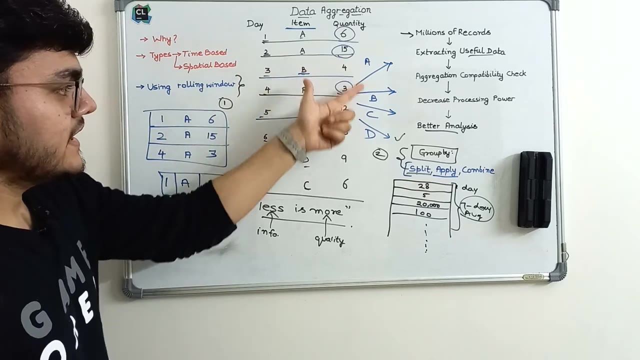 By taking the sum of all of these right. so six, seven, eight, nine, and here we have twenty four Right And the day is one right. so now you can see that I have simply splitted this data set into a, b, c, d, Which are the 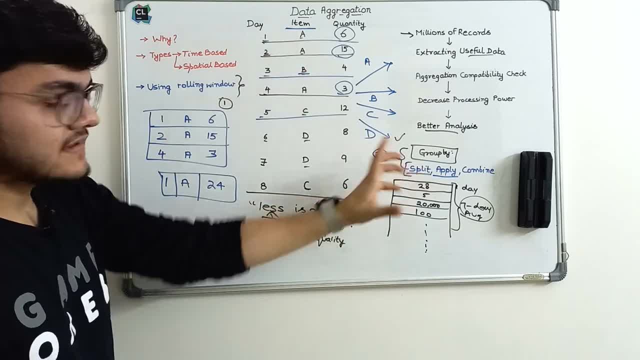 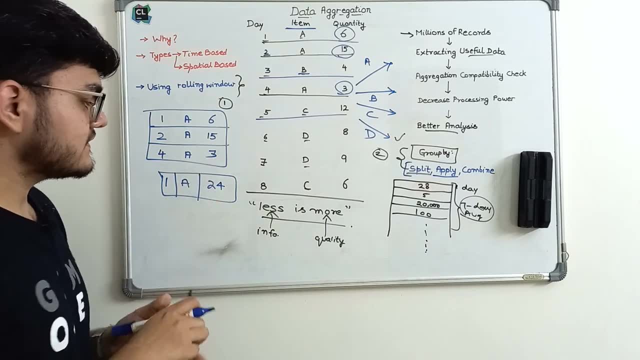 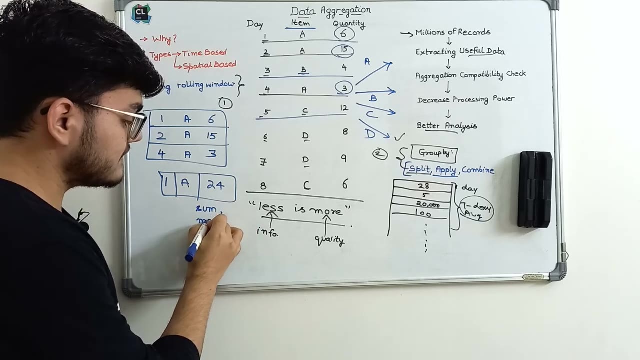 Categories and I've used a feature. so first task is splitting, then we are applying the aggregation. So there are different techniques you can use here. I have used some. There are some more techniques which we can use, like we have studied in statistics. we can use mean. 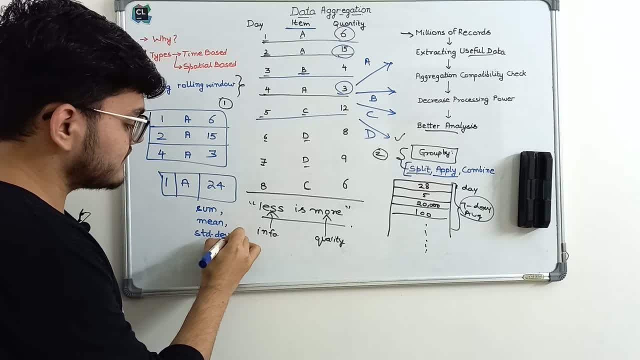 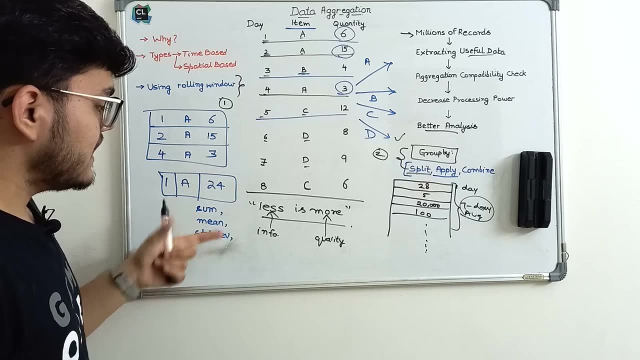 We can even use standard deviation to actually merge these columns. so what we can do is We can actually add them up and we can calculate the mean and the standard deviation, And then we will get the aggregated result right. so here we will get one result. 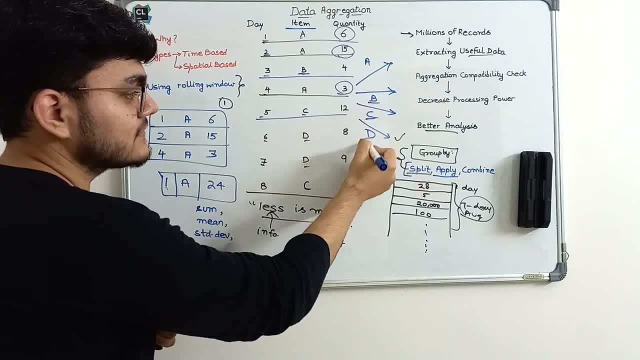 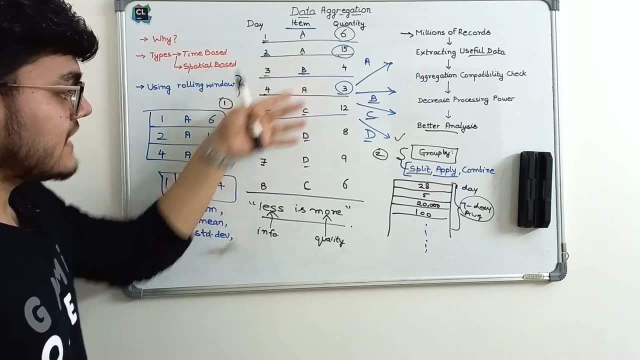 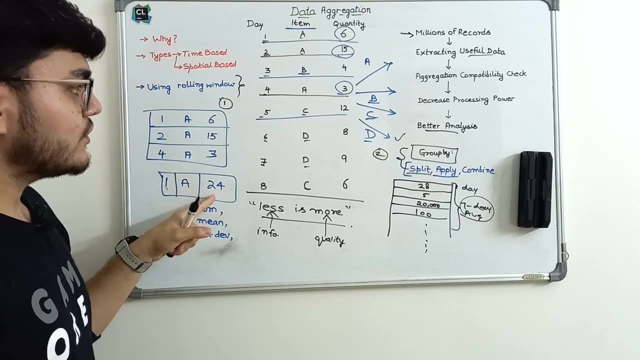 And similarly we can do with b, c and d also. so at the end you will see that there are four rows, Which is actually much lesser than eight. you can see we have minimized the whole data set, so now the data set is lesser. Plus, this is more practical because instead of seeing every day how a product is being sold, 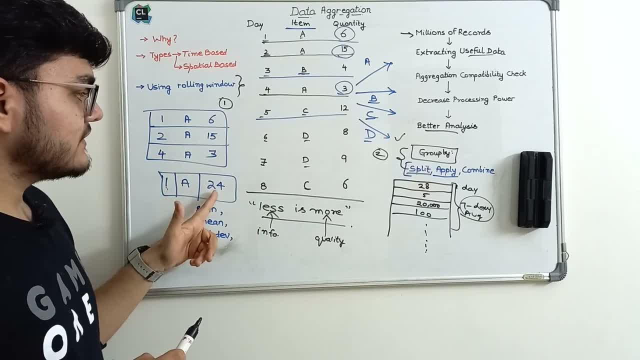 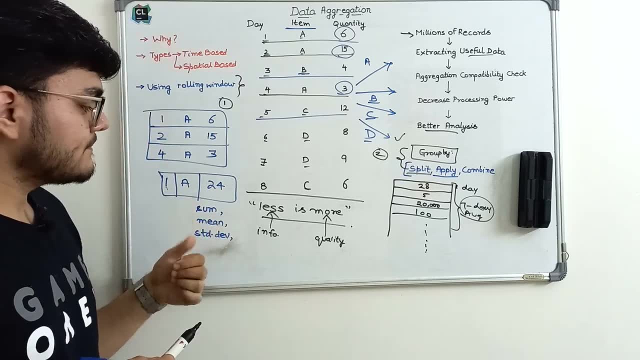 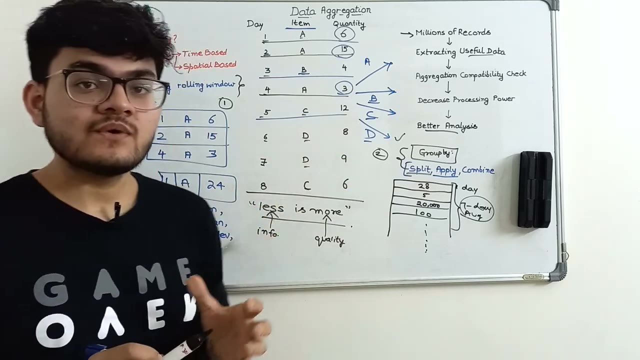 Now we know that this product, a, is actually sold in a. in eight days, twenty four products were sold right. So this is much more useful and much more meaningful for the business right. So it is important for a data scientist to understand the business logic first, because 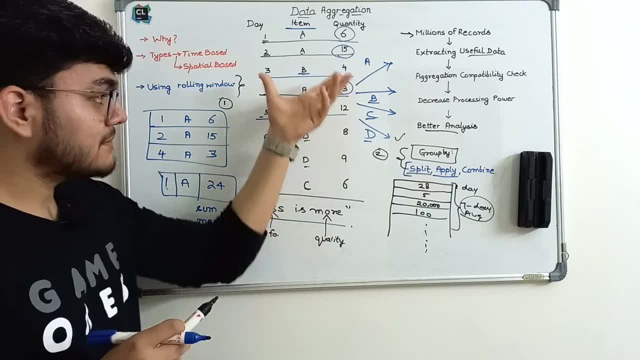 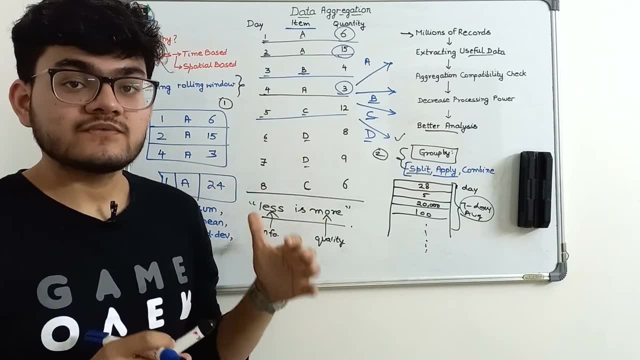 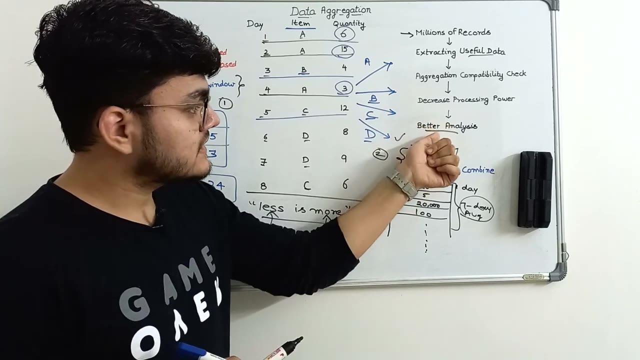 If you're applying some, it means that the act, the company which actually wants this data set, it is actually interested in All the number of the total number of sales of a particular item, right, And that is actually being passed to the better analysis. so the analyst will get this shorter data set. 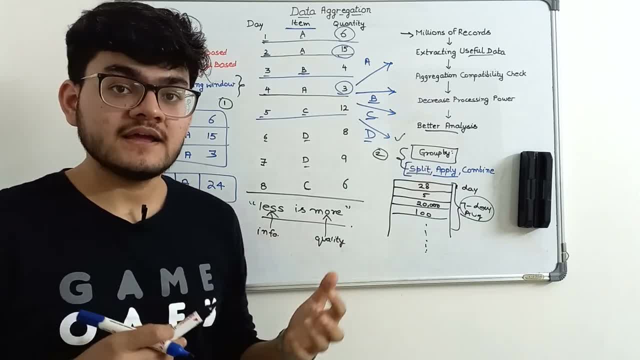 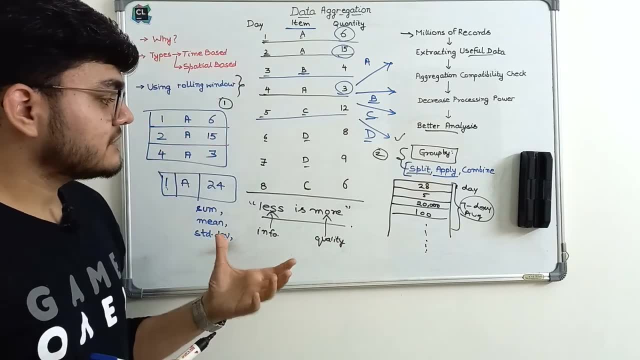 Which has less number of rows, but the quality is high, so plotting and doing things with that becomes easier, right? So now we're going to actually use python programming, where I will pick up a data set And we will use group by to actually do. 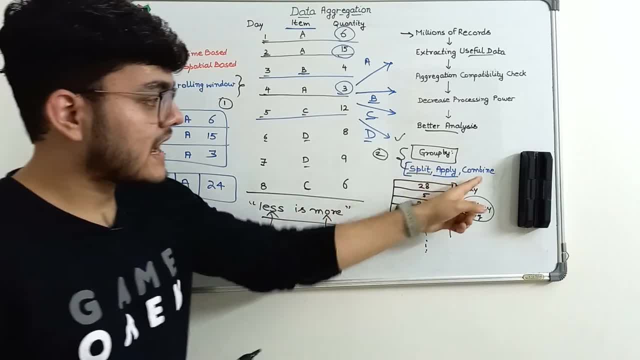 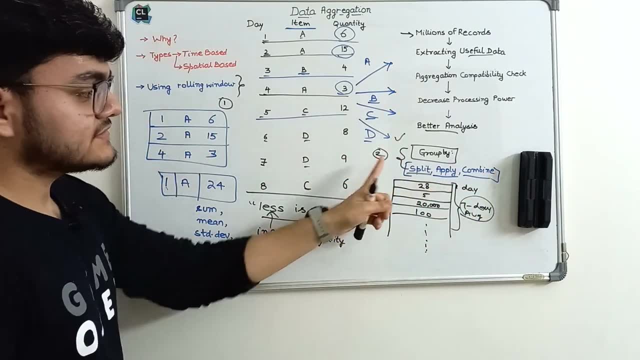 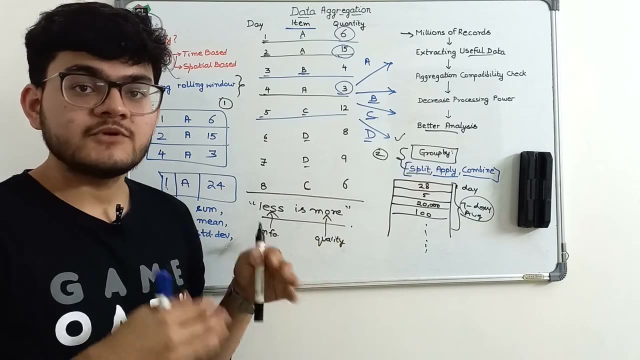 These two things, which is split, apply the concept, and then, finally, what we will do is we will combine all of them into a single one, Right? so this is one way of data aggregation: we split, we apply the operation and then we combine all of them to get up. 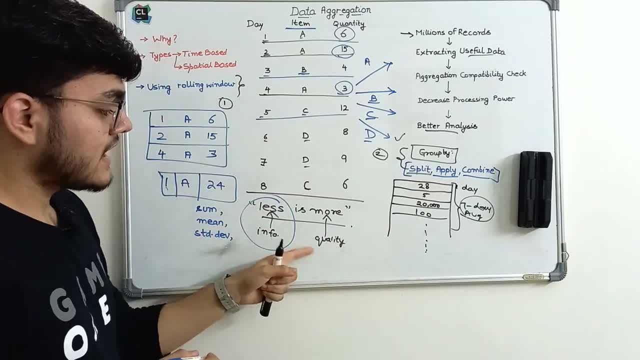 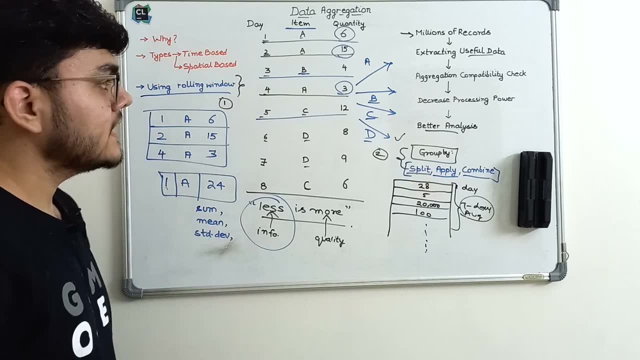 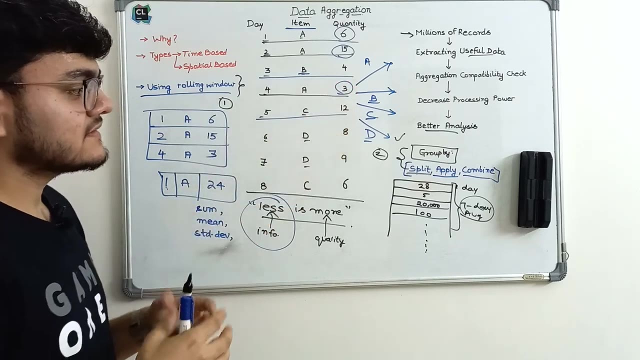 Shorter or a lesser data set which is having more quality. Now let's move on to this important concept here, which is using a rolling window. right, So now, instead of Using the item names as the number, as the, you can say, the criteria for aggregation, now we're going to use a rolling window. 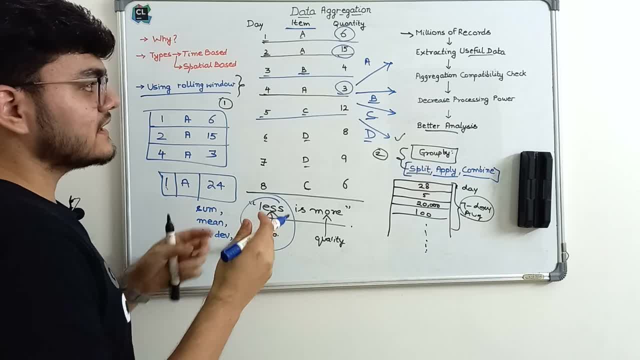 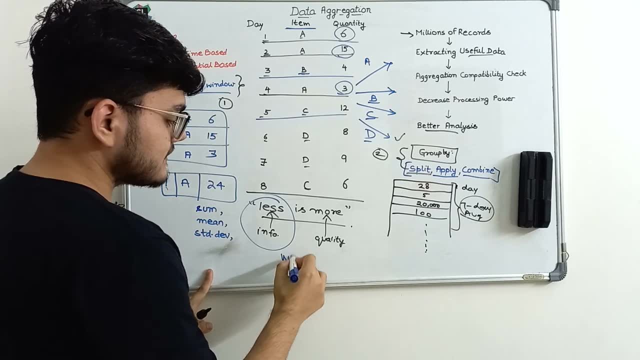 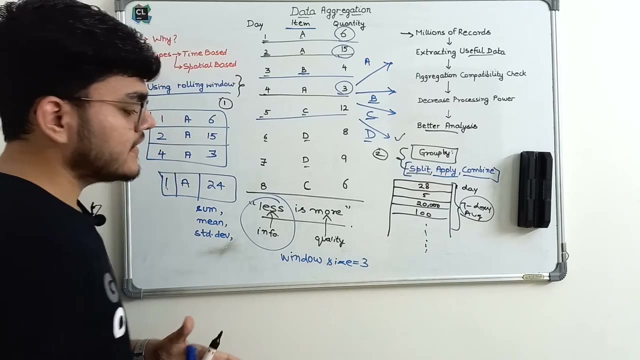 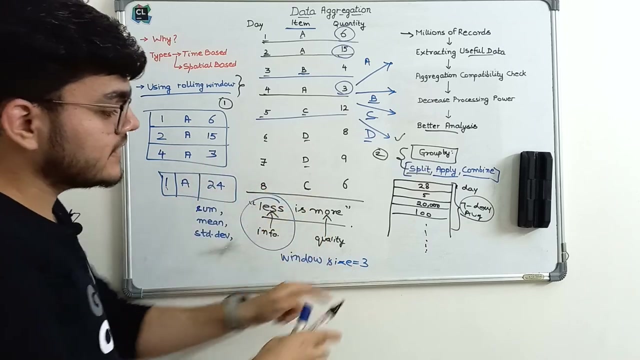 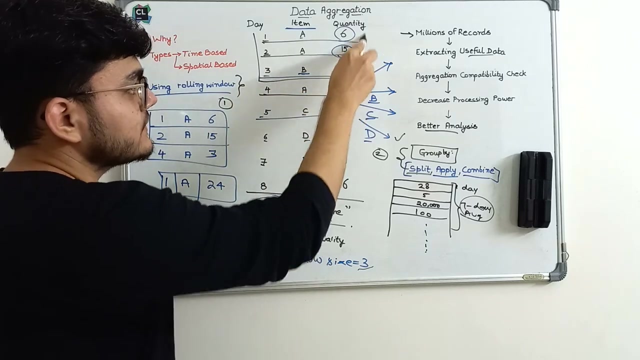 So what is a rolling window? rolling window is just like a window size, and first we will have to determine window size. So let's assume that the window size Is three, Right? so what are we going to do? is we're going to Imagine that we have a window that, at a time, can actually hold three number of rows, right? so here the window will start from, here it will actually point to the first three rows. 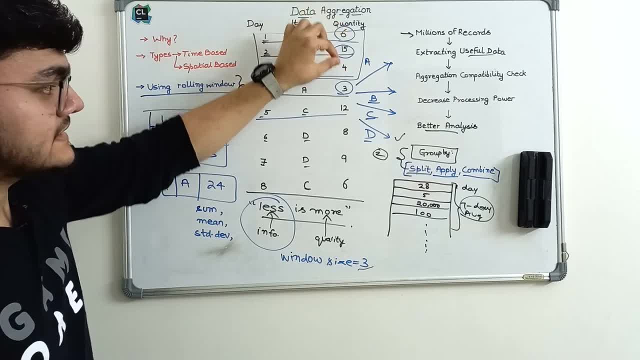 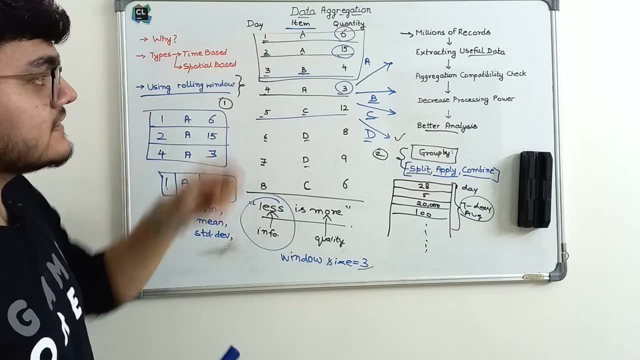 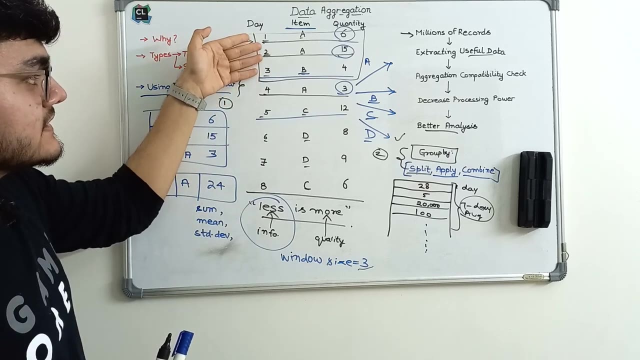 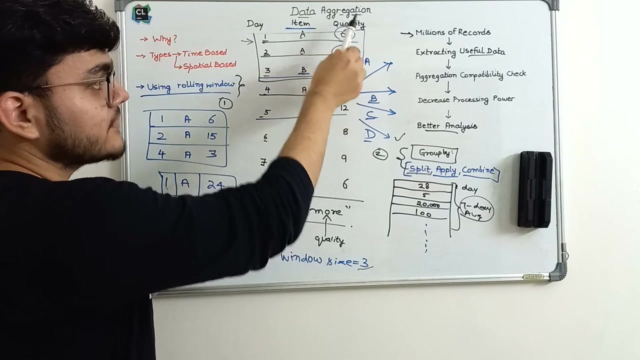 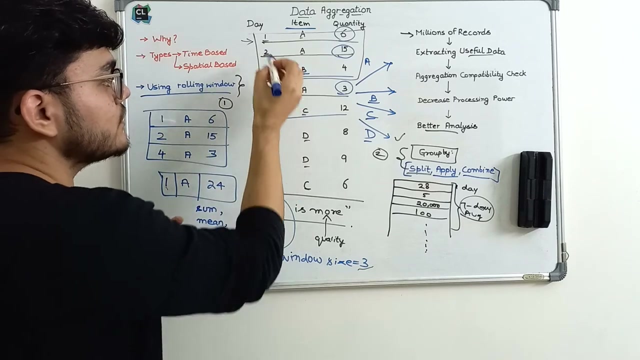 So this window. what it will do is it will calculate the, it will apply the data aggregation to these three rows and it will go and it will append the result in the first row. This is known as rolling window because, after Applying This concept, this window is going to roll one step ahead, right? so after merging these, after doing the aggregation on these three rows, what is going to happen is this is actually going to roll to the next one, which is like this: right? 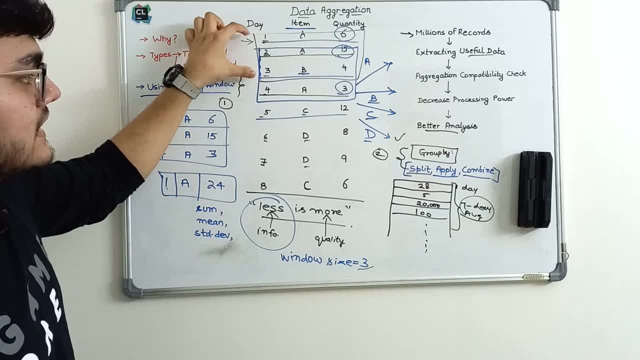 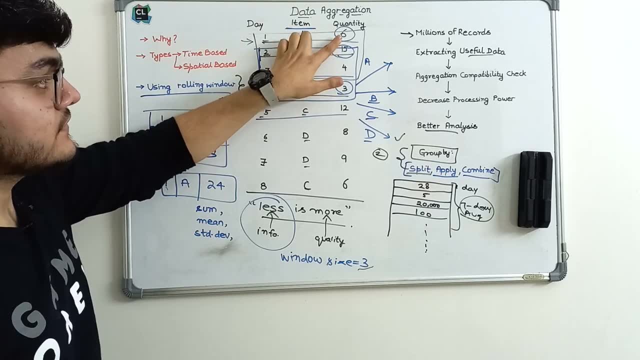 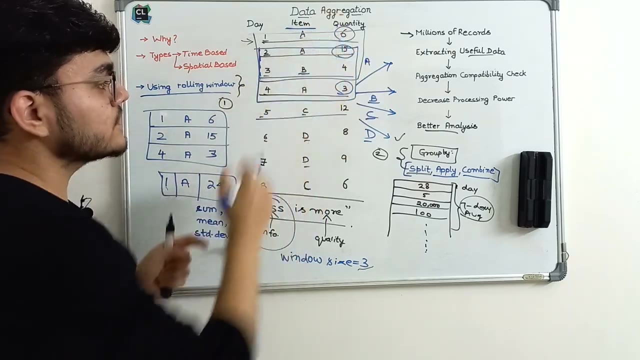 So first it will apply the aggregation on the first three rows, like you can say that, it will sum them up and you can see the sum is 19. Plus Six, which is 25, so it will append, it will override this with 25. so now, after doing that, the window will roll to the next record. so the next three items will be taken. 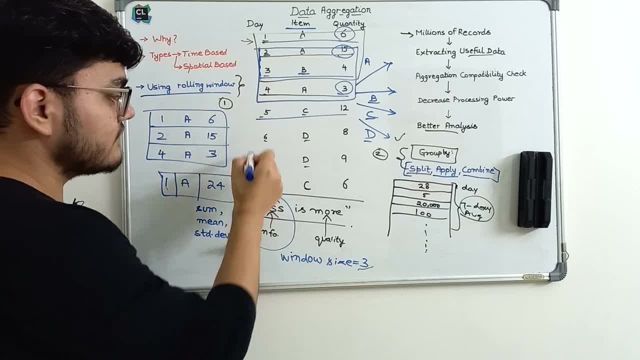 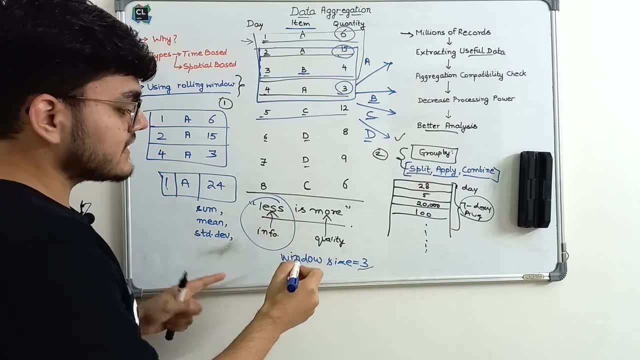 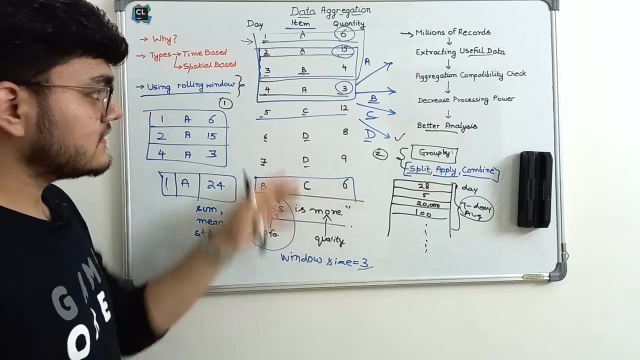 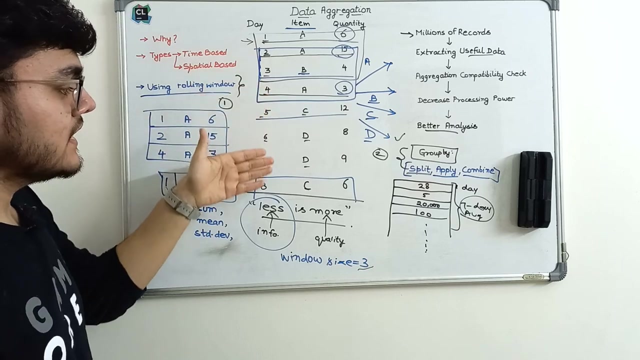 Again, it will keep doing this till the last one. so when it will reach the last one, we will have to specify a minimum size of this window. so if I specify that the minimum size will be a one, so when it gets one result- the Last one- this window will actually hold right. so we want a stopping condition so that we can stop this window from actually rolling right. this is the logical. this is actually the. 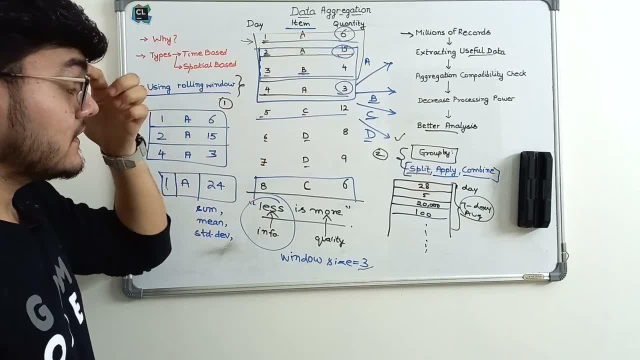 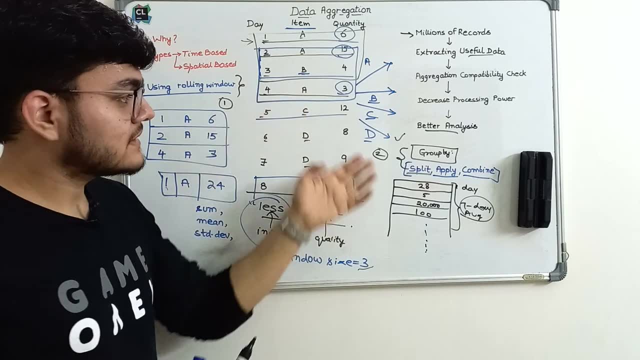 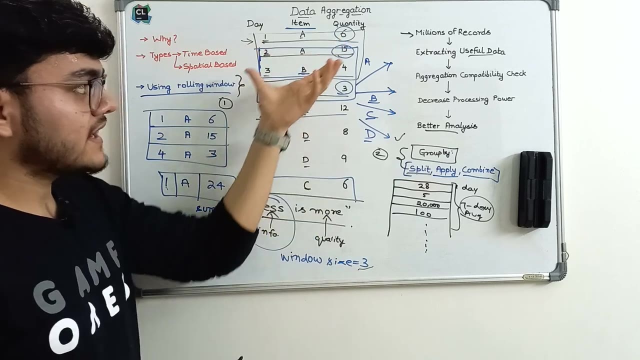 Idea behind it: aggregation, which is an, instead of using the group by, which is grouping. we are actually using a window size, so we are not discriminating in the item names. we are actually Using the rolling window to determine. determine that, all right. first i will take the first three rows, then next three, and so on, right.